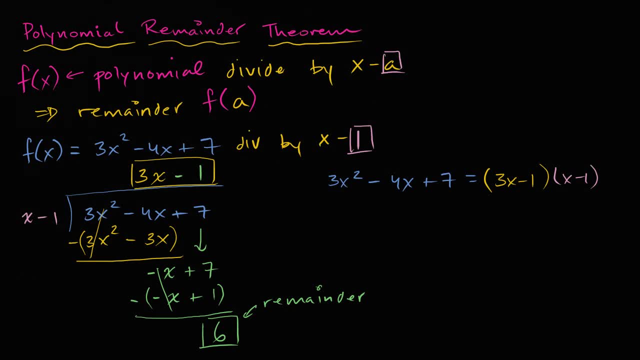 you're not going to get exactly this. You still have to add the remainder. So plus the remainder, And actually let me write the actual remainder down. So plus 6.. And the analogy here is exactly the analogy to when you did traditional division. 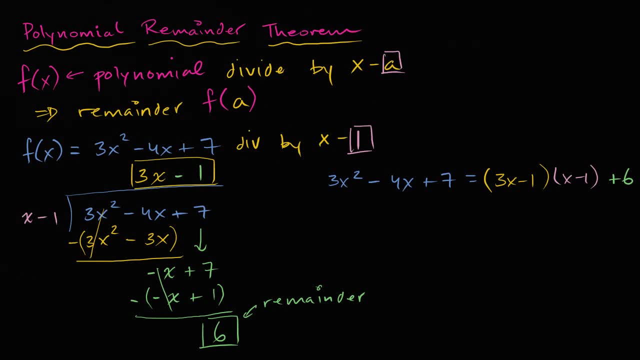 If I were to say, if I were to say: actually, let me just show you the analogy- If I were to say 25 divided by 4, you would say: OK, well, 4 goes into 25 six times. 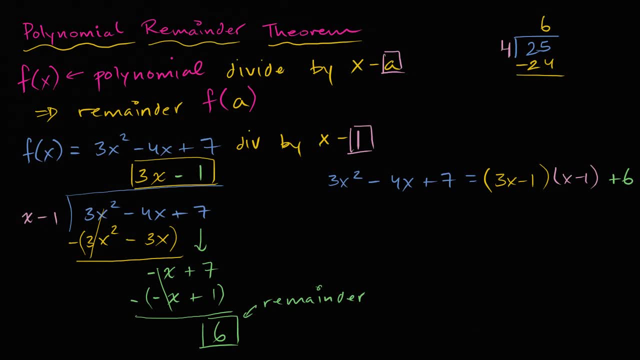 6 times 4 is 24.. You would subtract and then you would get a remainder 1.. Or another way of saying this is you could say that 25 is equal to 6 times 4 is equal to 6 times 4 plus 1.. 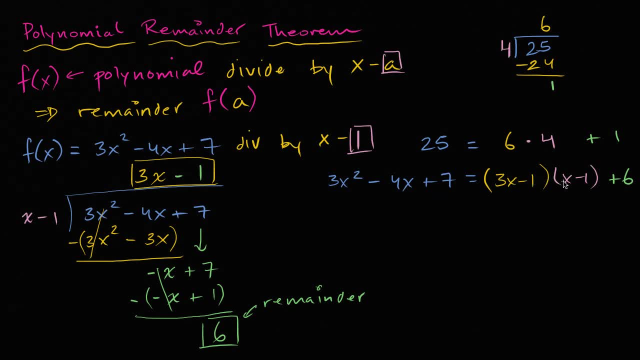 And so we just did the exact same thing here, but we just did it with expressions, And so, once again, I haven't started the proof yet. I just wanted to make you feel comfortable with what I just wrote right over here If I divided this expression into this polynomial. 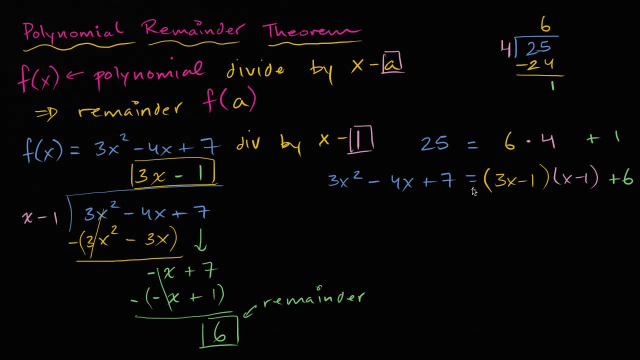 and I were to get this quotient, that's the same thing as saying: this polynomial could be equal to 3x minus 1 times x minus 1 plus 6.. Now, this is true in general. Let's subtract a little bit. 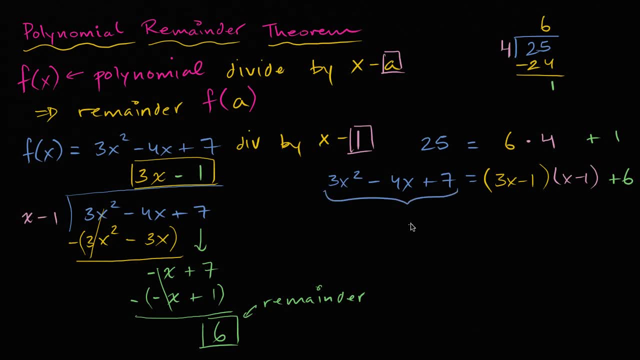 This is our f of x. So that is f of x. So that is f of x. So f of x is going to be equal to whatever the quotient is, And let me call that q of x. So this is a different color. 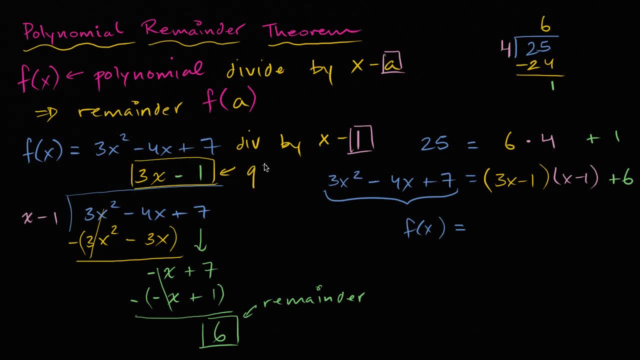 So I'm going to call that q of x, q of x. this right over here is q of x, So f of x is going to be equal to the quotient q of x times. this is our x minus a. in this case, a is 1,. 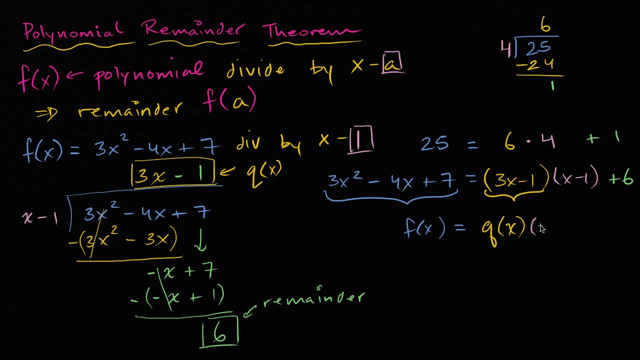 but I'm just trying to generalize it a little bit. So x minus a and then plus the remainder, Plus the remainder, And we know that the remainder is going to be a constant, because the remainder is going to have a lower degree than x minus a, and x minus a is first degree. 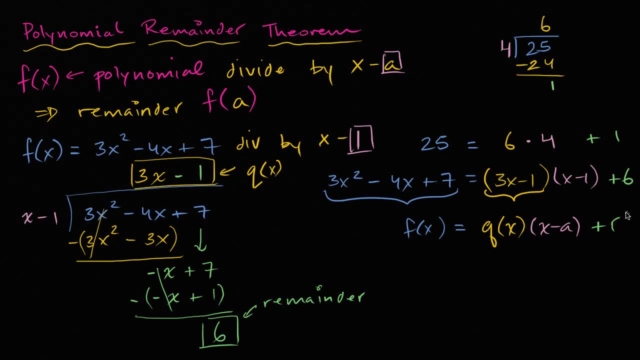 So this: in order to have a lower degree, this has to be zero's degree, This has to be a constant. So this is true in general. This is true for any polynomial f of x divided by any x minus divided by any x minus a. 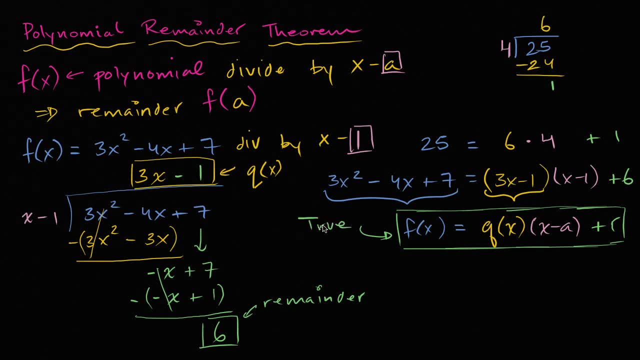 So this is just true. So this is true for any, for any, for any: f of x and x minus a. Now, what is what is going to? what is going to happen if we evaluate f of a? Well, if f of x is indeed, can be written like this: 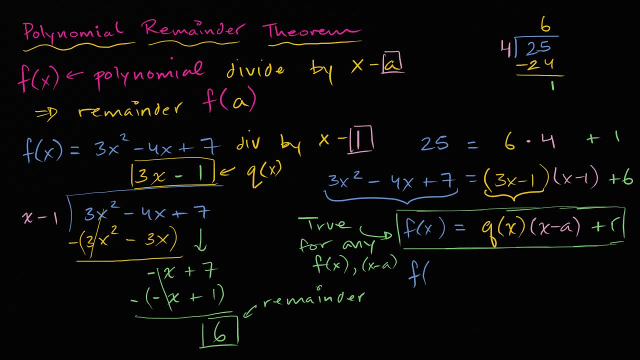 well, we could write f of- let me do a in a new color so it sticks out. We could write f of. a would be equal to, would be equal to q of a, so q of a, q of a times. I think you might see where this is going. 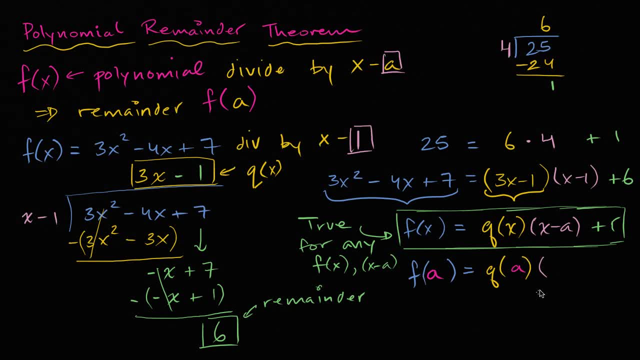 times a minus a times a minus a minus a plus r. Well, what's that going to be equal to? What's all this business going to be equal to? Well, a minus a is zero. So and q of a? I don't care what q of a is. 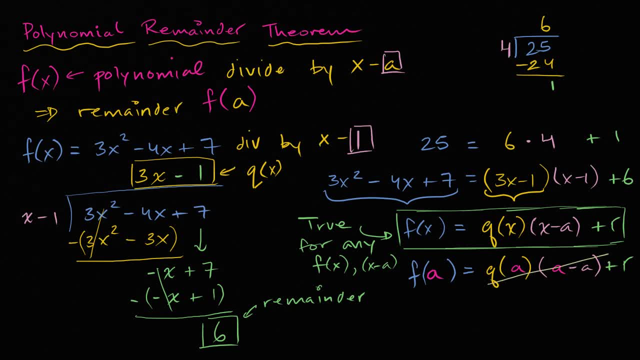 if you're going to multiply it by zero, all of this is going to be zero. So f of a, f of a, is going to be equal to, is going to be equal to r, And so you're done. This is the proof of the polynomial remainder theorem. 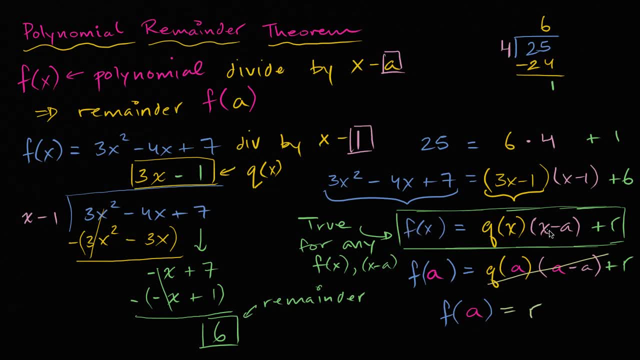 Any function. if, when you divide it by x minus a, you get the quotient q of x and the remainder r, it could then be written in this way. And if it's written in this way and you evaluate it at f of a, 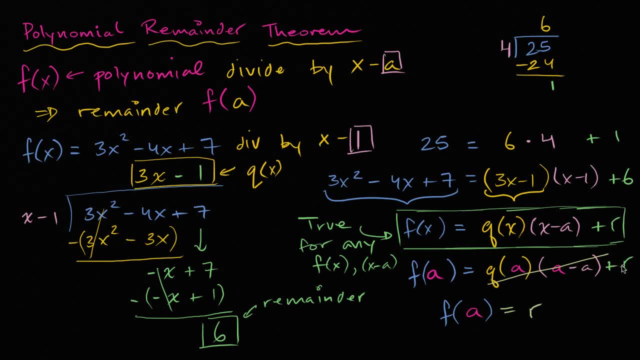 and you put the a over here, you're going to see that f of a is going to be whatever that remainder was, And that is the polynomial remainder theorem, And we're done One of the simpler proofs that exist for a, something that at first seems somewhat magical.